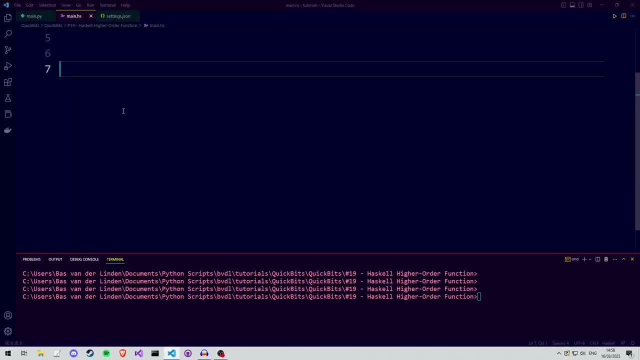 Hey everyone and welcome to this video going over an example of a higher order function in the Haskell programming language. Because Haskell is a functional programming language, it is common to use recursion in a function's definition, which makes for some elegant solutions. Let's take a look at our example higher order function called ApplyInOrder. 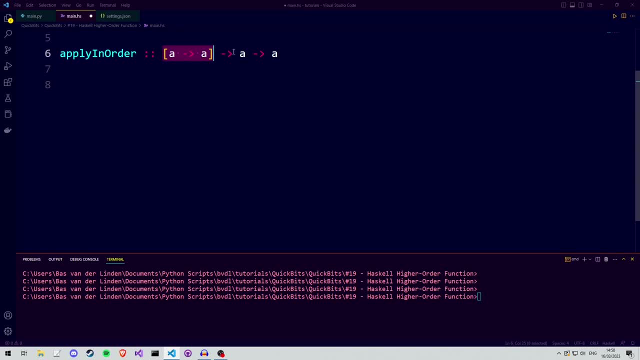 The function ApplyInOrder takes in a list of functions and applies each of those functions to a value x and then returns the result. As you can see, ApplyInOrder takes in a list of functions and each of those functions take in an argument of type a and return a value of type. 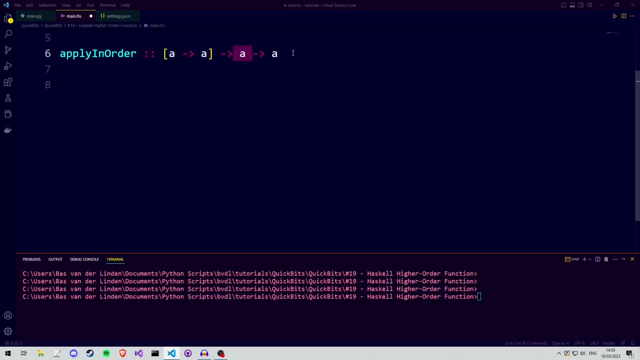 a ApplyInOrder takes in another argument of type a and returns a value of type a being the result of applying all the functions. Let's take a look at the base case of when the list of functions is empty. When the list of functions is empty and an x is passed. 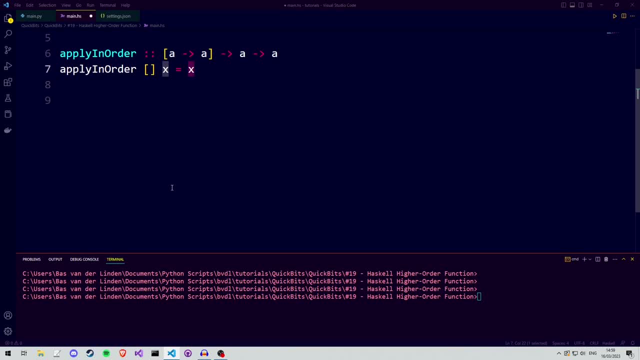 we return the value x because applying no functions to any value results in that value. Let's take a look at the recursive part of the definition. If the list that is passed is not empty, we return the value x, because applying no functions to any value results in that value. Let's take a look at the recursive part of the definition. If the list that is passed is not empty, we return the value x, because applying no functions to any value results in that value. If the list that is passed is not empty, we interpret the list as being f. 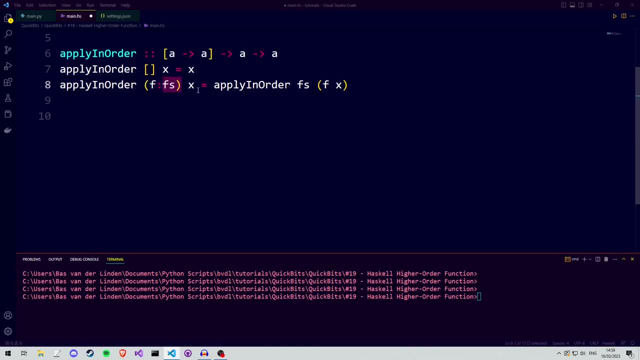 the first element in the list and fs the rest of the list and we also take in the value of x. As a result, we return the recursive function call of ApplyInOrder to fs being the rest of the functions, and as the new x, we return f applied to x. Now that the function is done. 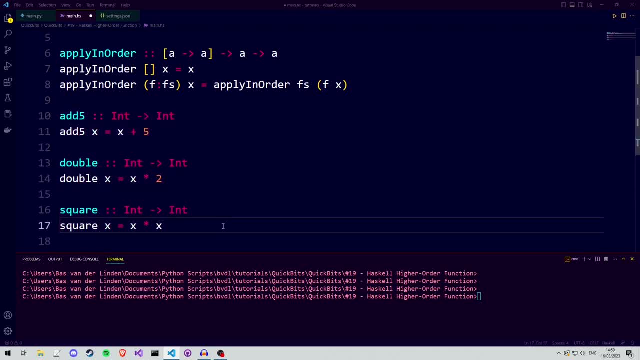 let's create three other functions which we can use with ApplyInOrder. We create a function add5, which takes in an integer and returns an integer plus 5.. We create the function double, which takes in an integer and returns an integer times 2.. And we create a function called square. 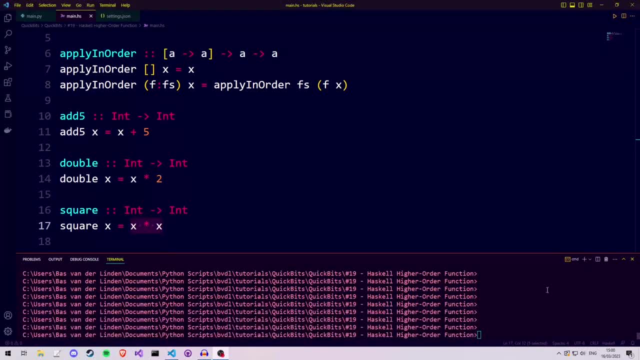 which takes in an integer and returns that integer squared. Let's load our functions into the Haskell interpreter by typing ghci, followed by our program filename. We see that the module was loaded correctly, so let's execute our function: ApplyInOrder. We execute ApplyInOrder, giving it add5,, double and square.